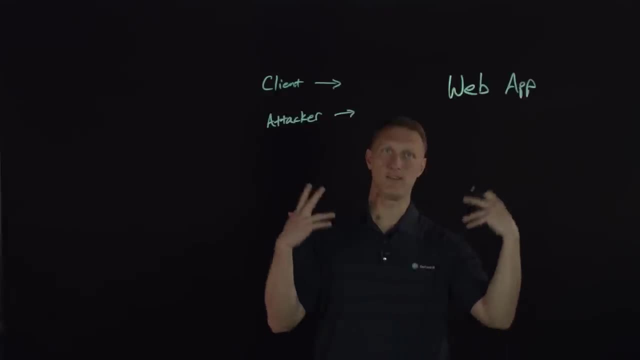 web application against these attacks. There's a couple of things you know from an overall security, you know approach that you can use to protect your web application, And the first thing that I'll mention is a standard, what we'll call a standard or network firewall. So let me put that down here. So I'll say 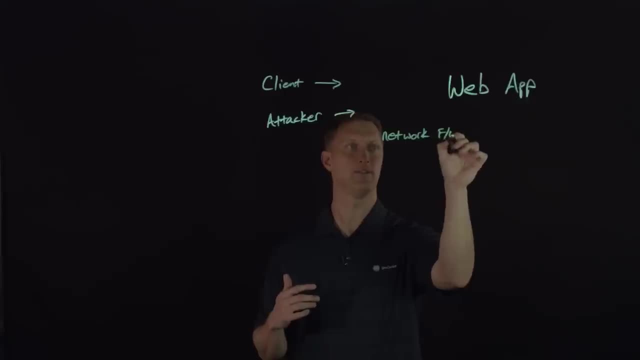 network and I'll just put FW firewall All righty. Typically a standard network firewall lives at layers, layers like three and four, And these you know. your typical network firewall is going to do things like IP protection, you know, from an IP address perspective, maybe like port, you know, protection, that kind of. 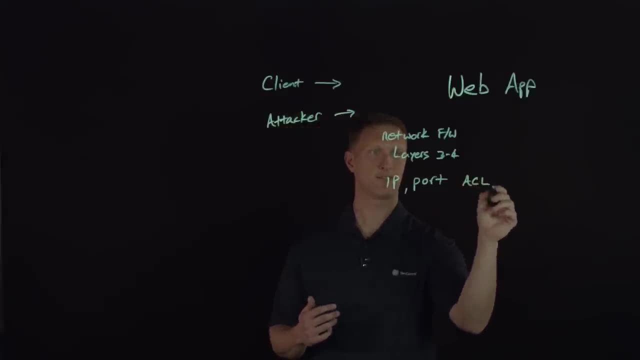 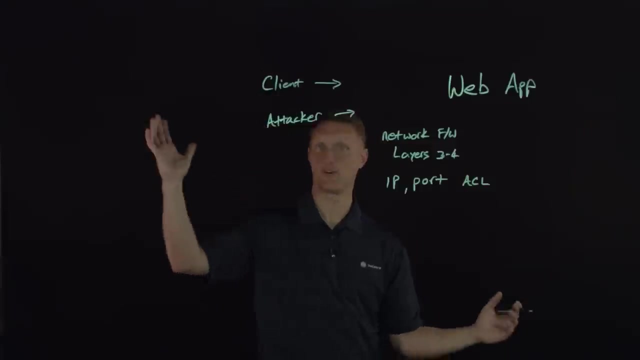 thing It uses. uses things like access control lists, ACLs. That is your standard network firewall. So if, if a client or an attacker, whoever it is, comes into your web application on IP address whatever or port number whatever as a destination, 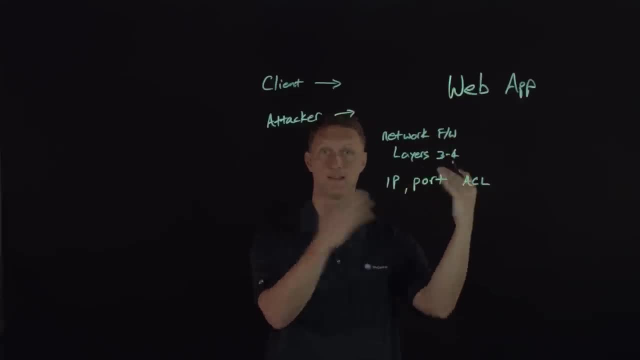 port, then your network firewall can block those, or they can let them in And your your typical layer three, four network firewall does a great job of handling that level of you know of access in your web application. More than just that, because there are other attacks that I'll put up here, and this is where a web application firewall comes into play. 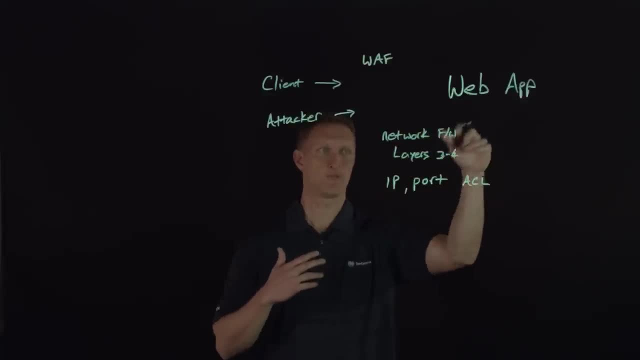 And these are at the higher layers, so, like maybe layer 4 through 7 or 5 through 7 is where the web application firewall lives and really does great things for you. So some things that a WAF would be able to help out with are things like, let's say, an HTTP flood attack, so I'll put flood up here. 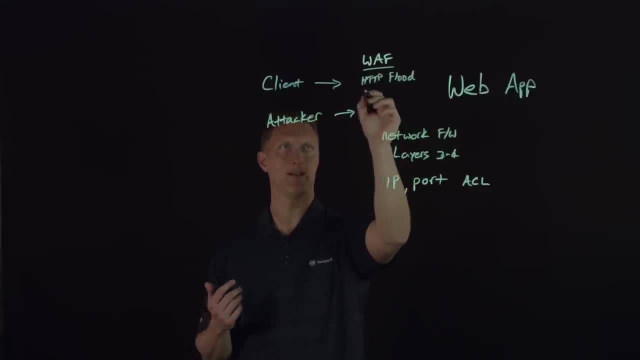 There's another attack- and these are some specific things that I'm mentioning right now. I know, but you can understand- in general, Things like slow loris is a specific attack that would come in at the higher layers on your web, On your stack, that a traditional network firewall is never going to be able to block or would just would not block based on what its functionality is. 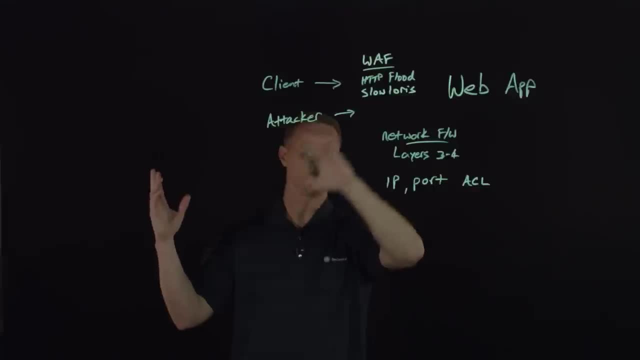 All righty so, from a like an HTTP flood, for example, or a slow loris attack. these are attacks that present a legitimate HTTP request to your web application. It's going to pass through any network firewall, I mean, given that it's on, you know, an IP and port that's allowed through the firewall. but let's say that that's true. 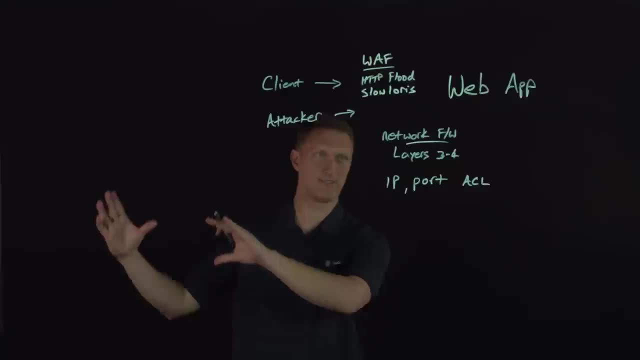 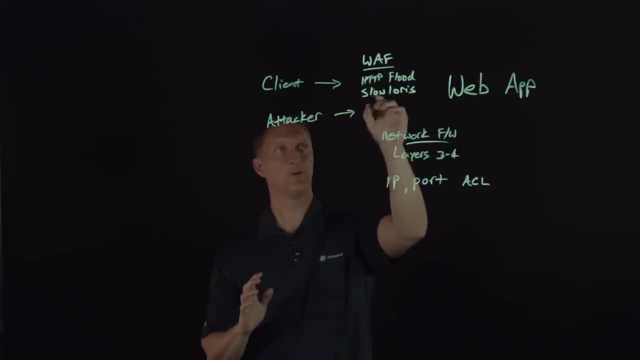 Then, Then, the actual nature of the attack itself is not to attack the network itself, but rather to attack the web application. So again, these are legitimate HTTP requests that are coming specifically at your web application that a traditional network firewall is not going to stop. 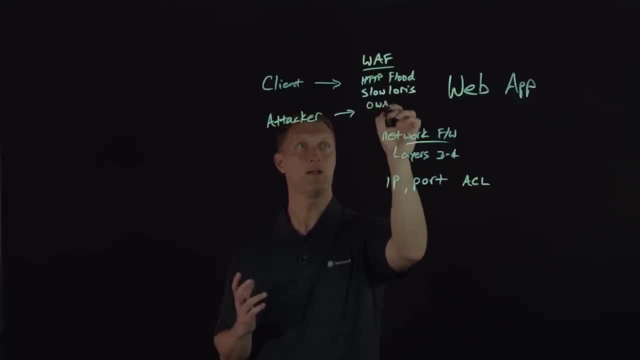 I'll also put- let me put OWASP, OWASP top 10 up here. All righty, The OWASP top 10, and we did a whole series on these. There are things like injection attacks, cross-site scripting. There's 10 of them. 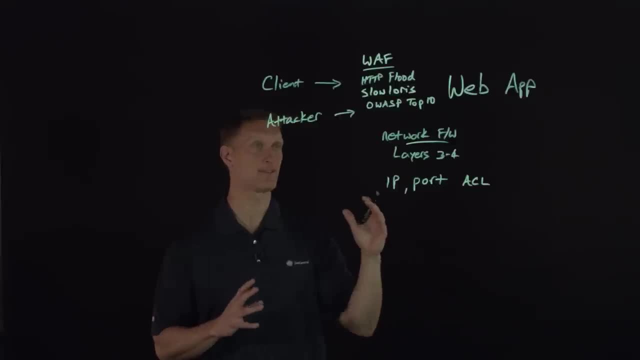 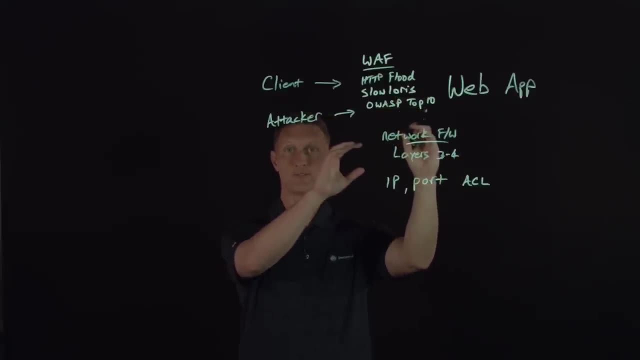 You know there's, there's, there's a lot of these that are out there, these security risks, And the the web application firewall is frankly designed to look at those types of security risk on the OWASP top 10 and to mitigate as many of those as possible. 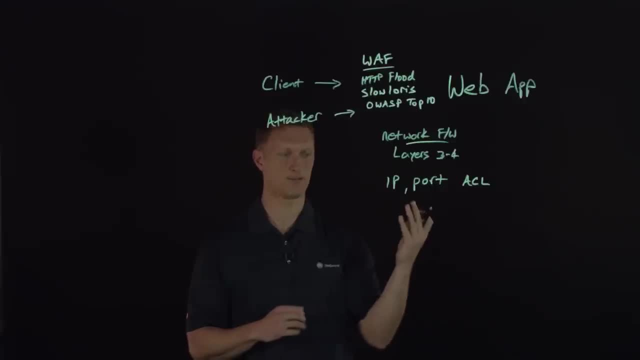 It can't mitigate all of them, because some of them are like the number 10. one is insufficient logging and monitoring, So that's where you just need to log your stuff or you need to monitor your application. You need to make sure that you're monitoring your applications properly and so that so it doesn't it doesn't stop. OWASP is not going to stop every one of the top 10, but it's going to do a great job at most of them. 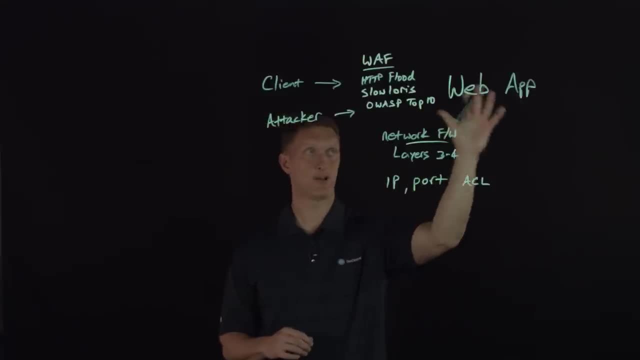 One of the other things that I would mention is: you know, when you talk about web application security, the the ultimate answer in terms of someone that would say: well hey, why do I even need a web application firewall? Obviously, what I just mentioned is true. 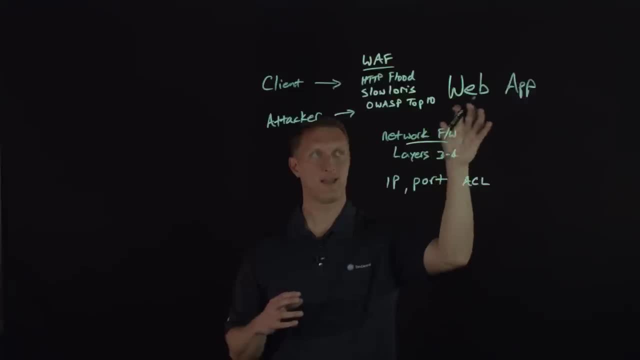 The. the fundamental answer, though, is you need to design and build Your web applications securely. So if, theoretically, if you did that, if you design your web application securely, where a cross site scripting, you know attack- were to try to happen, or an injection attack or some sort of untrusted user input was going to be, you know, brought against your web application and do some nefarious thing, then if you built it correctly, then you could try to, or you could. you could block a lot of those just by designing and building your web applications. 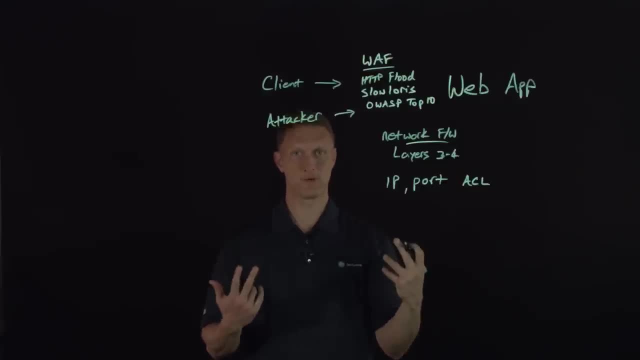 Properly, but we live in the real world today and there are a lot of applications that are just not built properly or their legacy applications that, even though they did a great job at the time they were built, things have moved or things have progressed and they're not secure anymore. 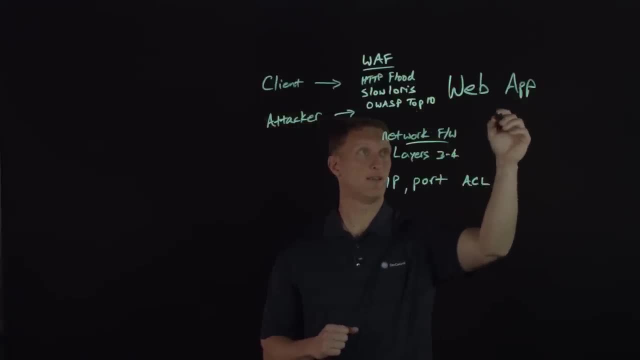 So instead of just maybe one web application, let's say you know you have. let's say this is a representation of your web application. Let's say you have, you know, a hundred of these things. back here, You got tons of them that you have to protect. 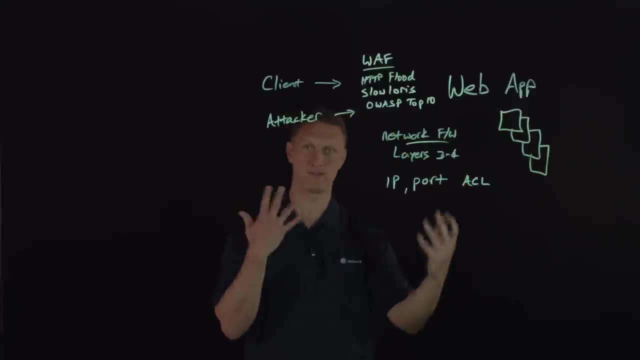 And each one is designed differently. Each one is, you know, handled separately all that kind of stuff. So how in the world are you going to take every single one of your, your unique web applications and modify those, configure those, and all that so that they can handle all of these higher layer attacks that would be launched against them? 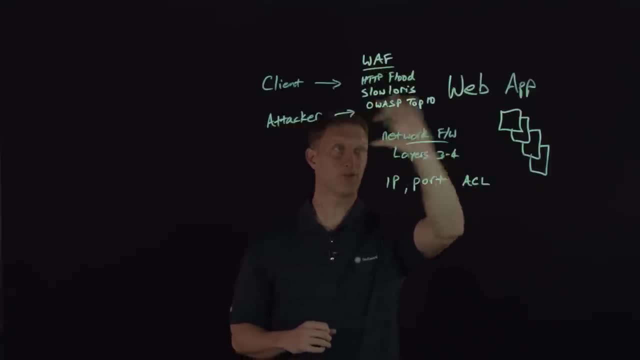 And the answer is: if you put a WAF or a web application firewall in front of the web applications, then you can configure the web application firewall And it will handle all of the The attack stuff against all of these applications. you don't have to go back there and handle all of these separately. 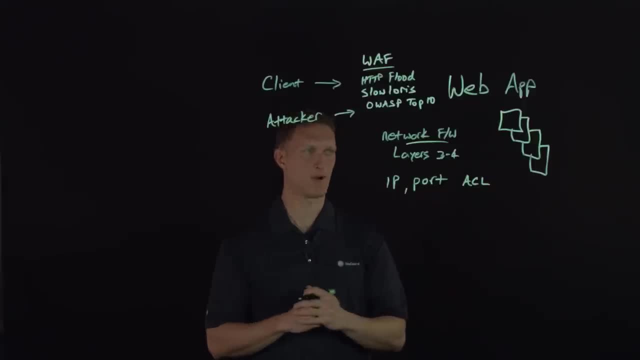 Ideally, of course, you do want to make sure that they're, that they're configured properly, and all that, But but anyway, but that's that's one of the reasons that you would need a WAF as well. So one other thing that I'll mention is the HTTP protocol that our web applications today just live and die by is was never really designed for the complex web applications that we have. 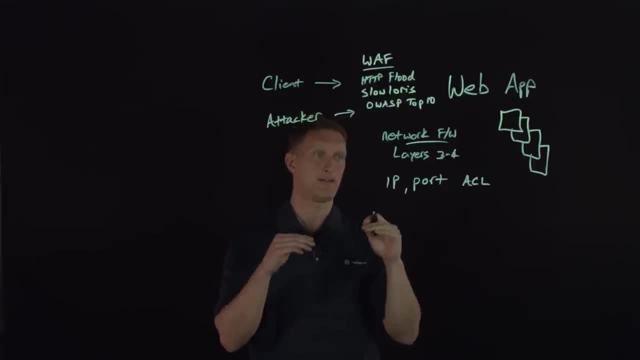 We have in play today. So, while you might say, well, hey, let's just handle this at the protocol level, at the HTTP level, Unfortunately, HTTP, you know what it was designed. it was not designed with, Again, these complex applications in mind. 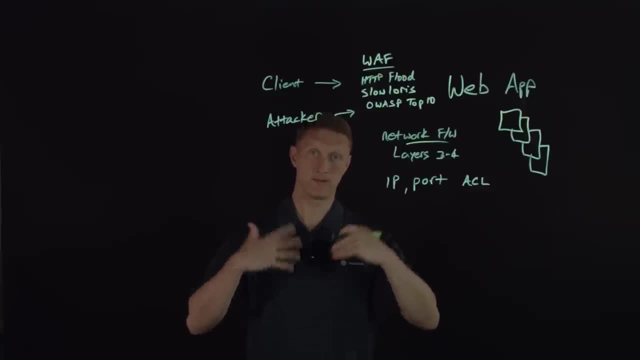 And so there are fundamental protocol level vulnerabilities or, or you know, weaknesses, as it were, that can be exploited Again. that's where a web application firewall can come in and say: hey, as a, as a what would have been a. 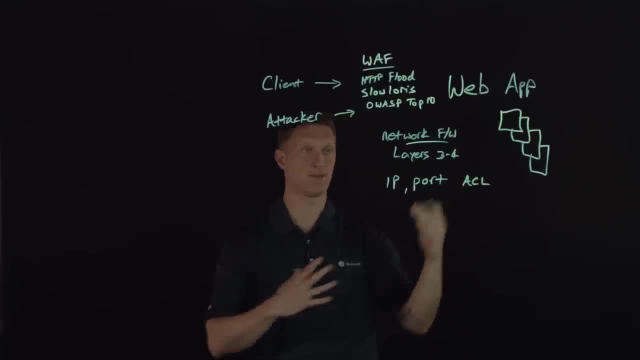 Legitimate, legitimate HTTP request coming into my web application. as that comes in, I'm going to inspect that. I'm going to check it out. make sure it's not an injection attack. it's not a cross-site scripting attack. it's not a HTTP flood or slow lures or any number of things.